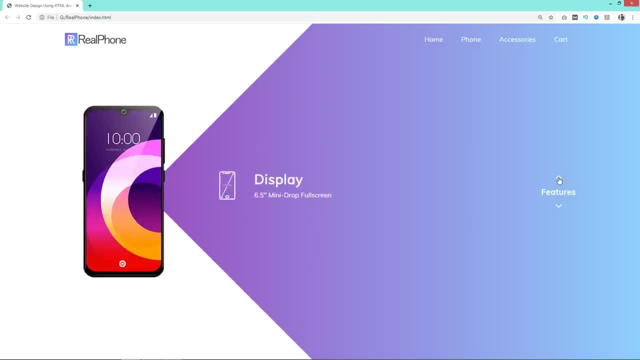 i click on up arrow, it will rotate the content in anti-clockwise direction. in every click it rotate the content and display another feature of this phone. this click and rotate function is made using simple javascript that i will teach in this video. you will learn to make this complete design in. 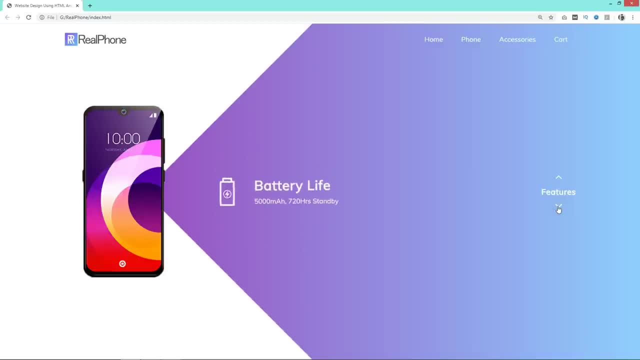 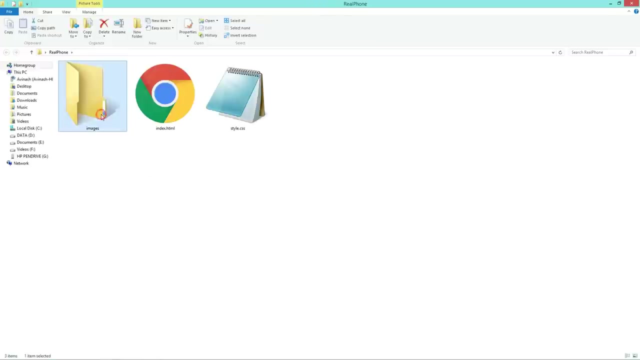 this video step by step, so don't skip this video and keep watching till the end. before starting, please hit the like button and subscribe my channel. if you are new here now let's start this video here. i have one folder and in this folder i have one html file and one css file. i have one. 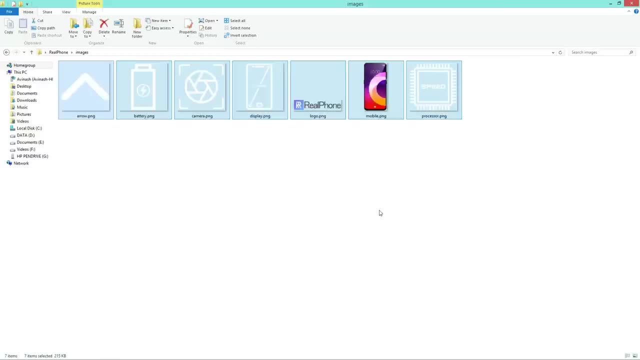 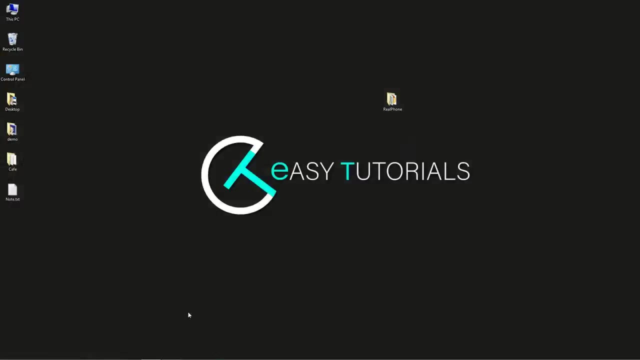 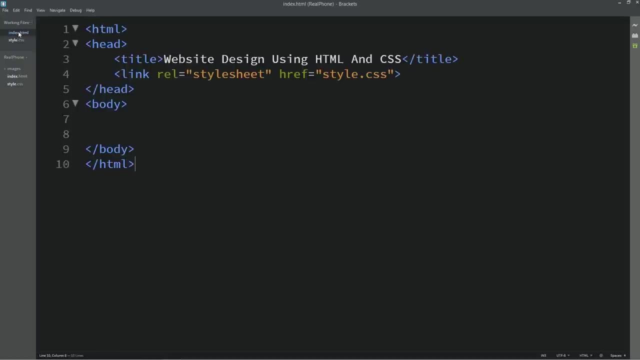 more folder here and in this folder you can see some images and icons. now i will open my text editor, which is brackets editor. so this is our html file. i have written written basic html structures and this is the css file. you can see i have connected html file with css with this line of code: 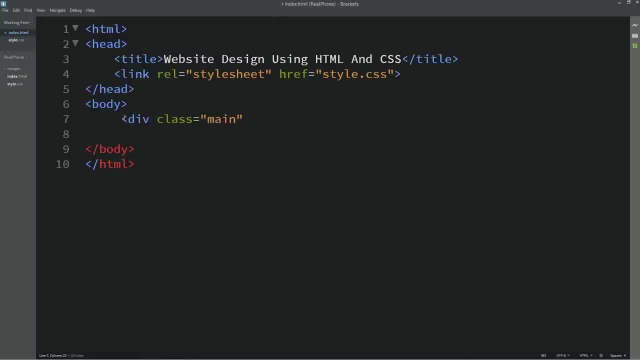 next we will come to the body tag and here we will create one division with one class name and the class name i am adding main. let's copy this class name and add it into the css file, and for this one we will add: the width and height. position will be relative and overflow. 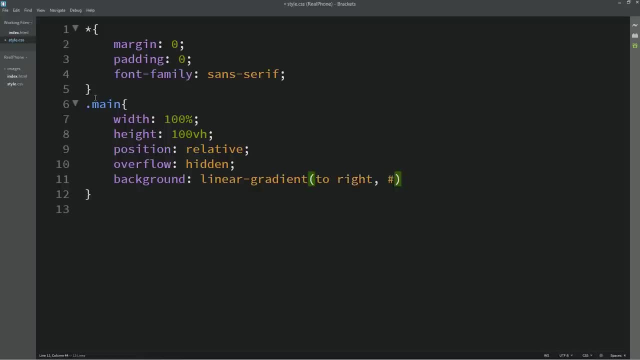 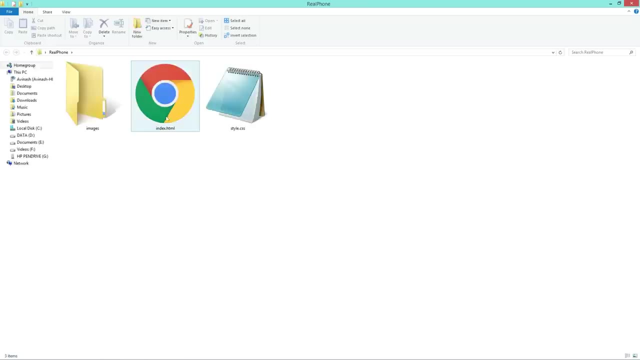 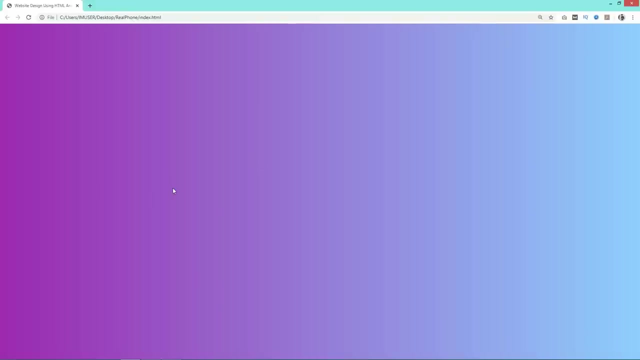 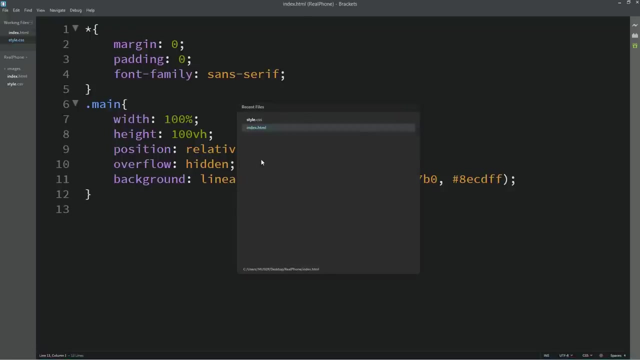 hidden. we'll add linear gradient color in the background. let's open our html file with google chrome so that you can see this gradient color on this complete web page. let's come back to the html file and here we'll create one tag nav and in this nav will add one division and one class name. 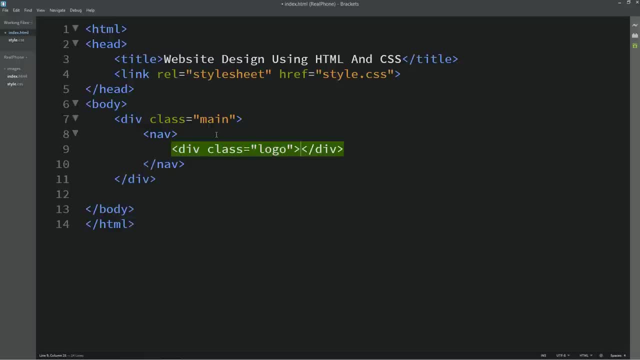 in the class name i am adding logo. simply duplicate it and change the class name. nav links: we have two div here. in the first one we'll add logo image. so for the logo image you will have to open your microsoft browser here and the picf. 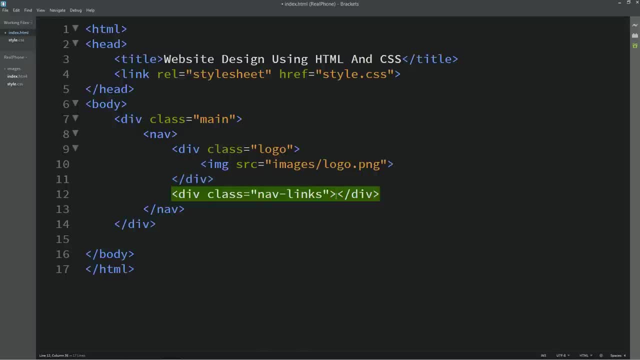 i am adding img source and the image file path. in the next div we'll add ul and li to create the navigation menu. here we are adding href for the anchor tag. simply duplicate it and add different menu title. so the second one is phone, next is accessories and the next is cart. 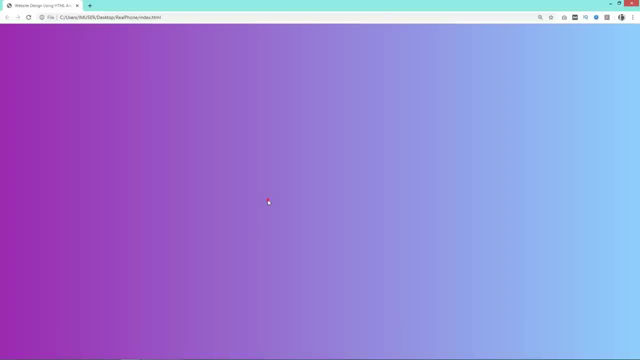 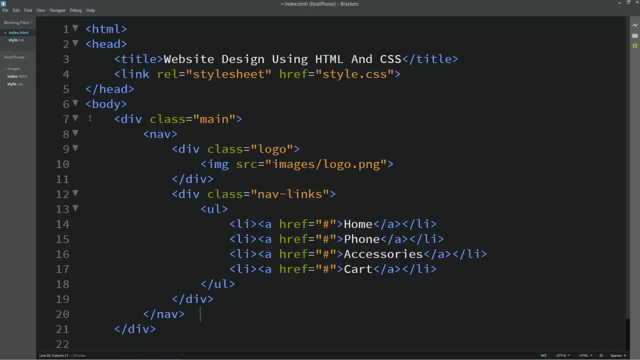 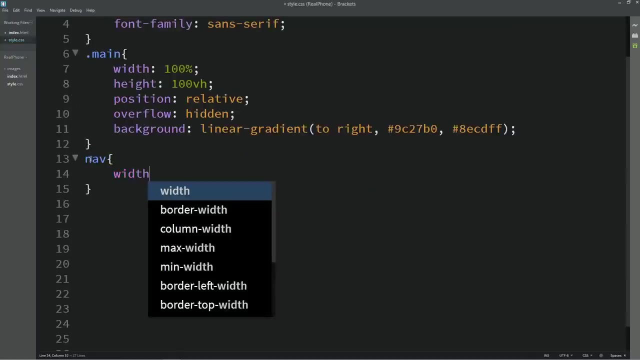 let's reload the web page and you can see this logo and some menu at the top. let's come back to the html file. copy this nav, add it into the css file. here we'll add width, then position sticky margin: 20 pixel and auto set index: 1. display will be flex and align item center. 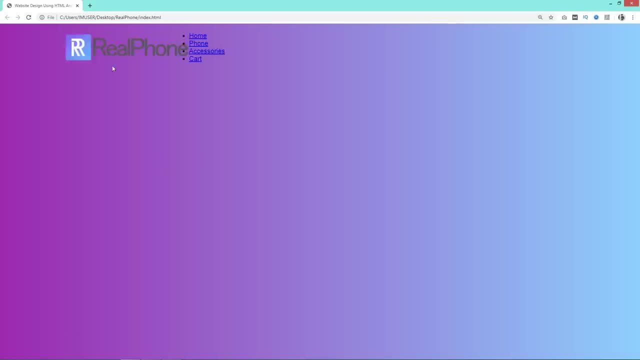 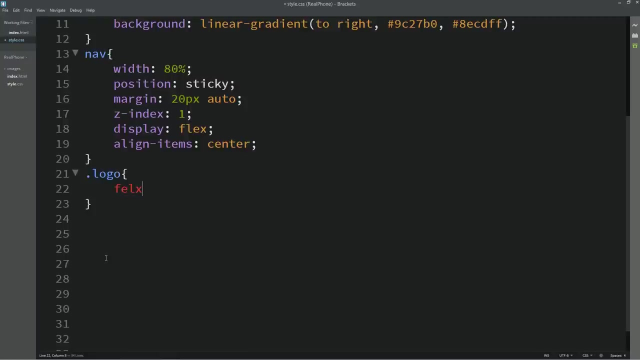 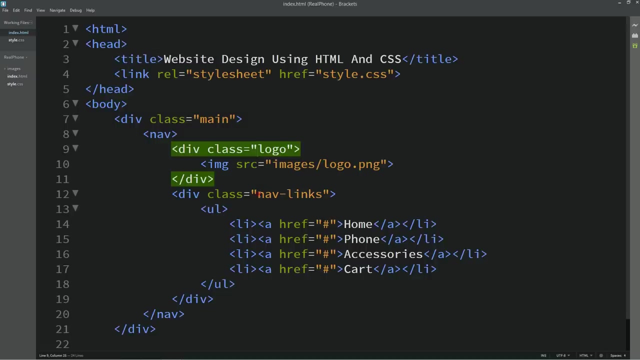 let's come back to the html file. copy this class name logo, write it here in the css file, and here we'll add flex basis 20. just copy it again, then write img, and for the image we will set the width. next, copy this class name nav links, write it into the css file, and here we'll add flex 1. 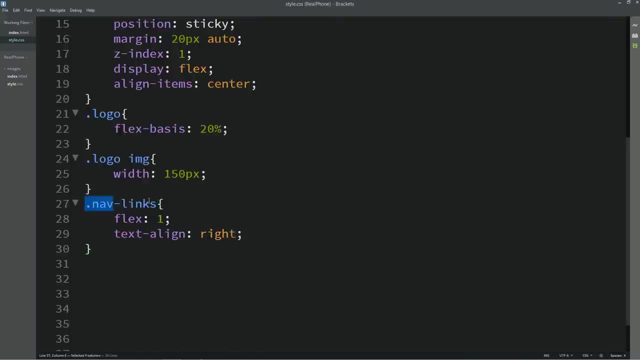 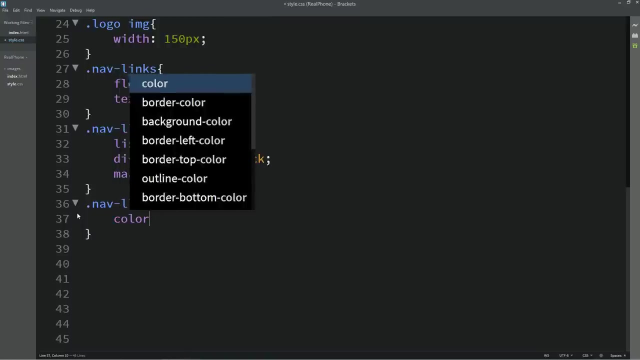 text align right. just copy it again. then write ul and li list style: it will be none and display: it will be inline. block margin: 0 and 20 pixel: just copy it again. then write a for the anchor tag. here we'll set the color and text decoration. 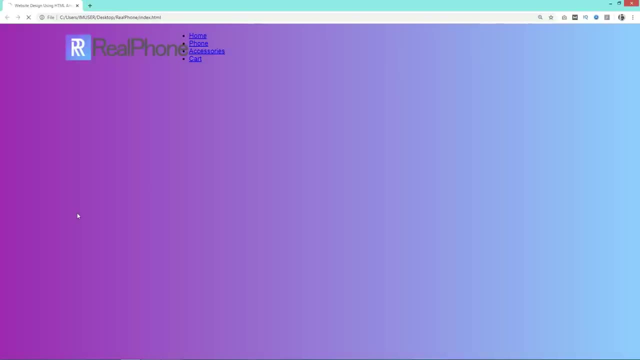 it will be none. refresh the page and x and tick inflammation. it works. it's gonna work. based also once item and run github, your github app. Then type Where is cool wonder and tap 틴 page and you can see these menu on the right side. 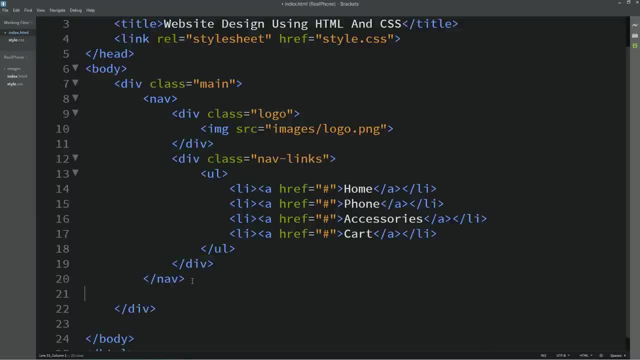 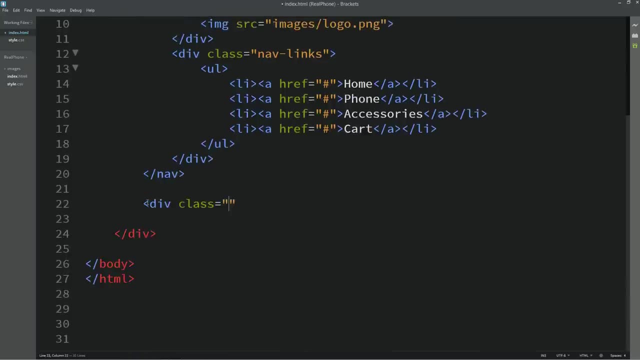 Let's come back to the HTML file, and after this nav we'll add some content. So first we'll create one division and we'll add one class name. I'm adding information. Let's add one more division here and we'll add one ID circle. 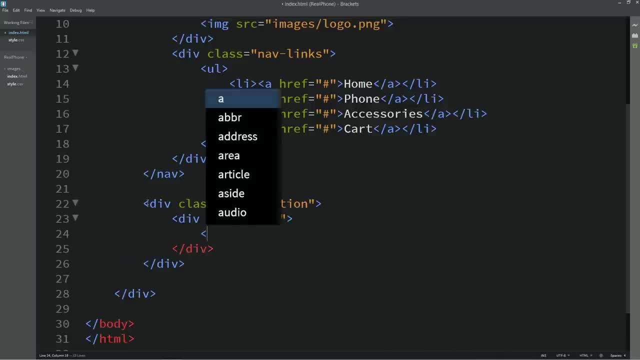 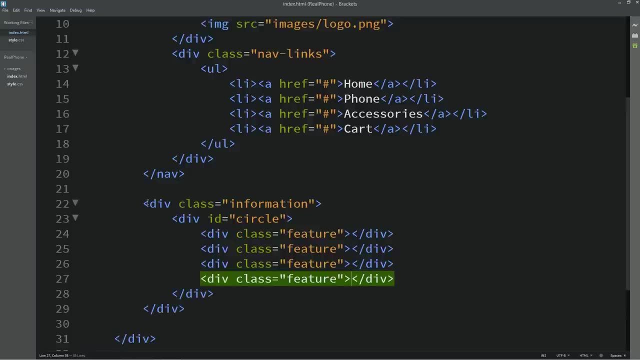 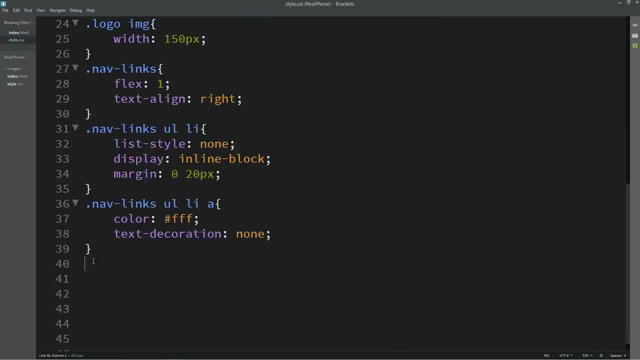 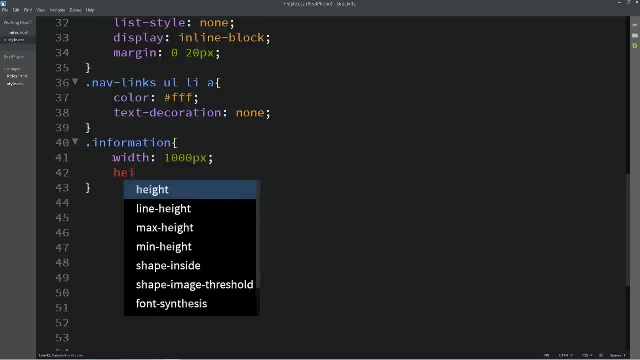 In this div. I'm creating a div with the class name feature and duplicate it because we will add multiple features here. So just copy the first class name, write it here in the CSS file information. here we'll add width And height. 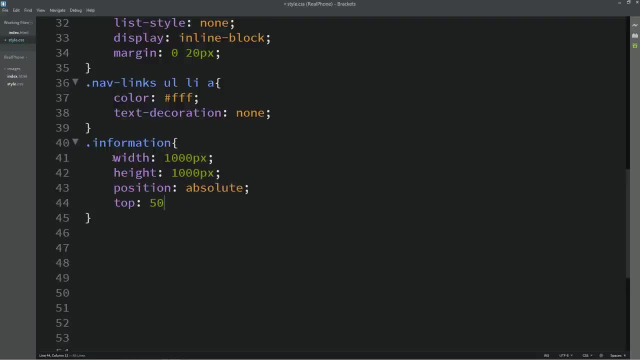 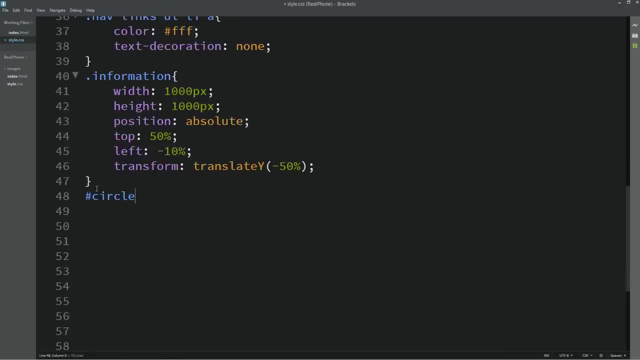 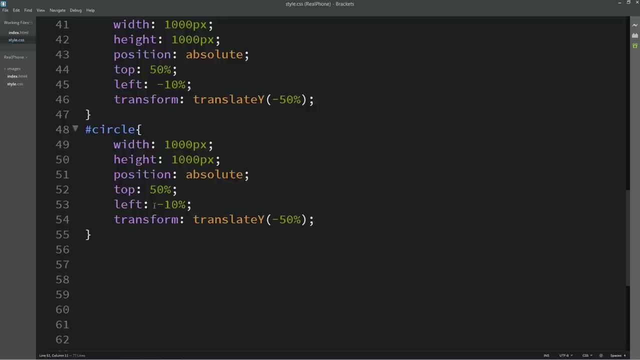 Then position: absolute and top 50%, left minus 10%. transform translate y minus 50%, So it will be vertically centered. Let's copy this ID circle, write it here. Just copy everything here. We will change this top and left. 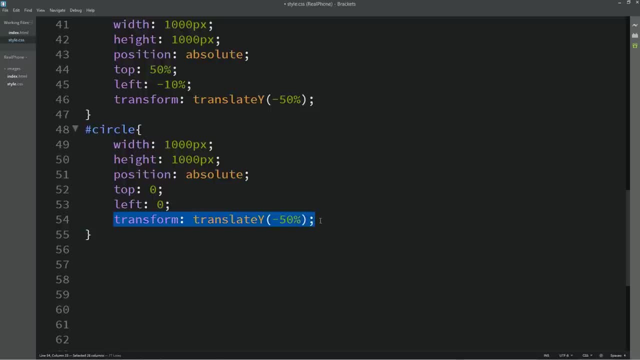 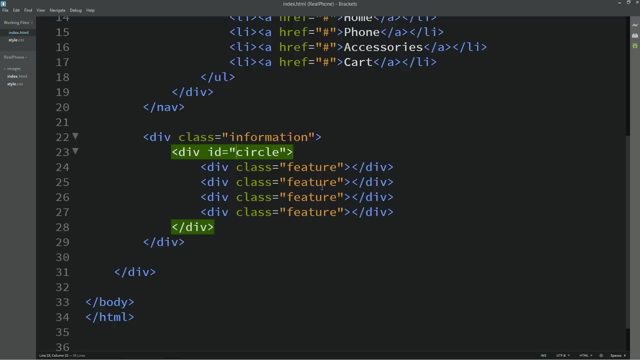 Remove this transform and here we'll add border radius. It will be 50% because we are creating one circle. Next we'll add background: It will be gray. Refresh the web page and you can see this circle in the left side. Let's come back and in the first feature we'll add one icon. 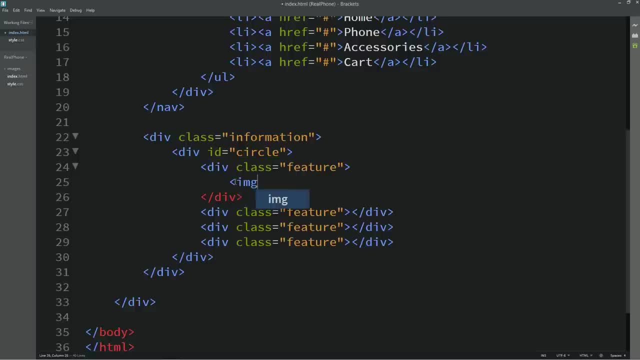 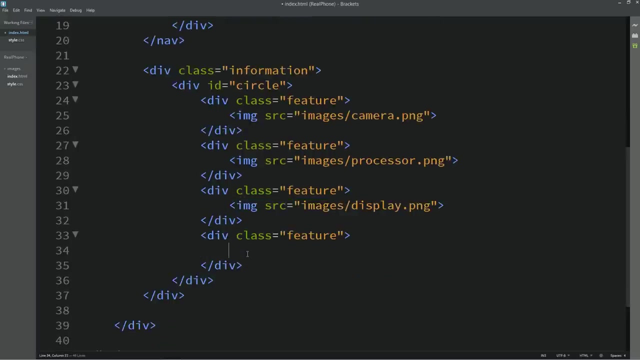 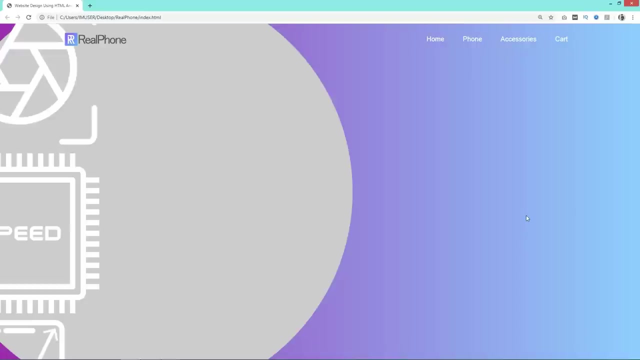 Sorry, Icon, So I'm using img source and the image file path. Simply add it in the other one. also Here we'll add different image. In the third one, Again different image, and now in the fourth one, Refresh the web page. 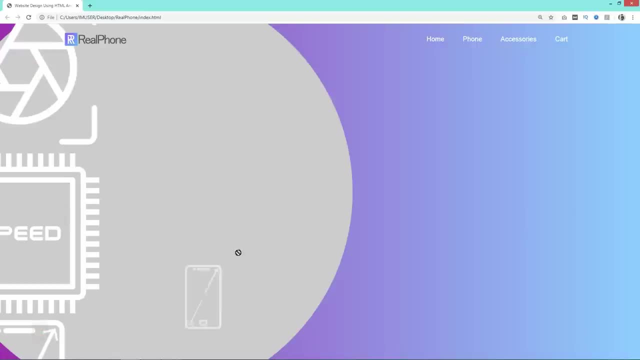 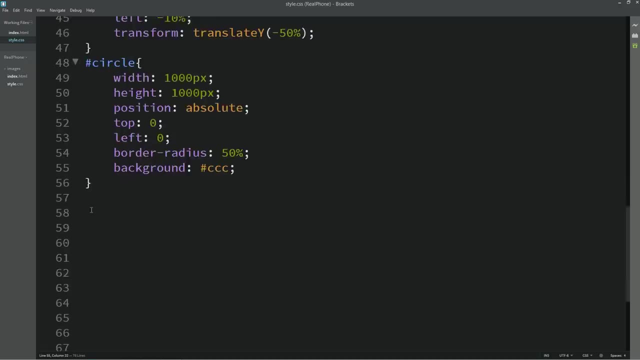 You can see these icons on this web page. We have to change its size and position, So just copy this class name feature, write it here, Then write img. Here we'll add width: 70px. Again, write feature and position will be absolute. 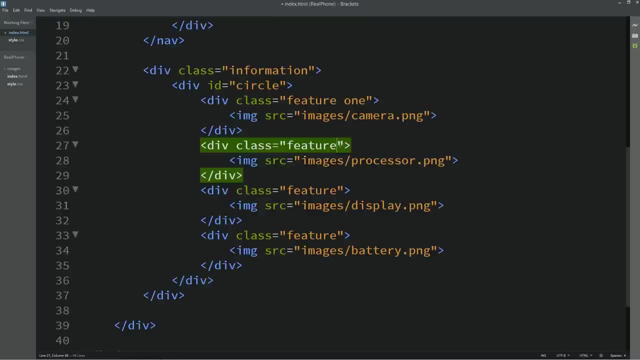 Now in the each feature we'll add different class name. So first I'm adding one, in the second one, Two, Three and here we'll add four. Use the first one, Write it here, because we need different position for each images. 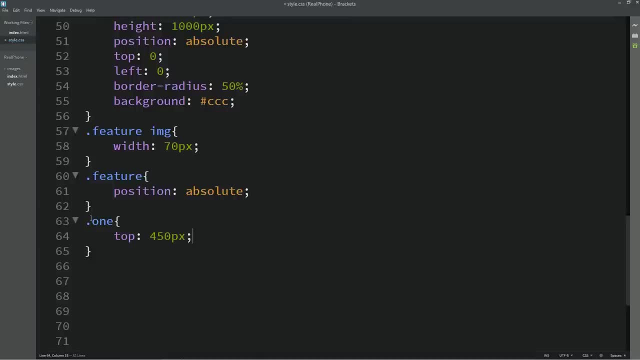 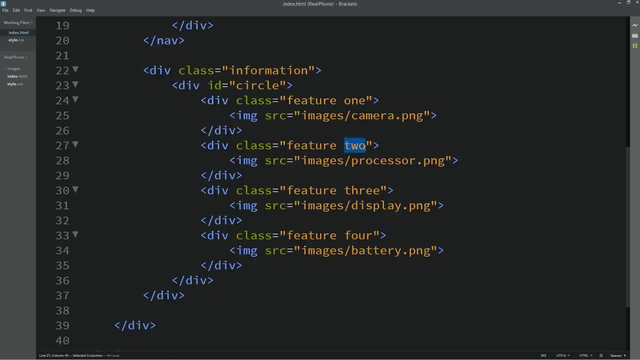 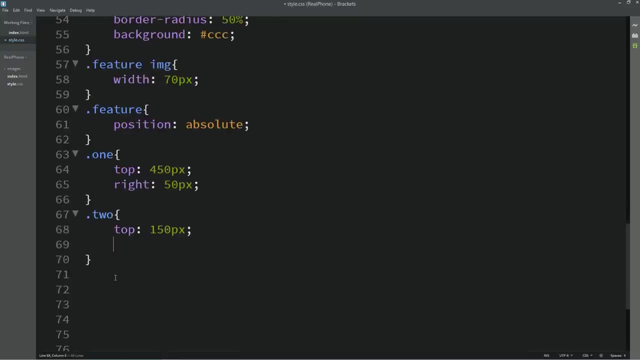 So here we'll add top 450px and right 50px. Now we'll copy the second class name. That is two. Here we'll add different position from top And from left. Now for the third one. Here I'm adding bottom and left. 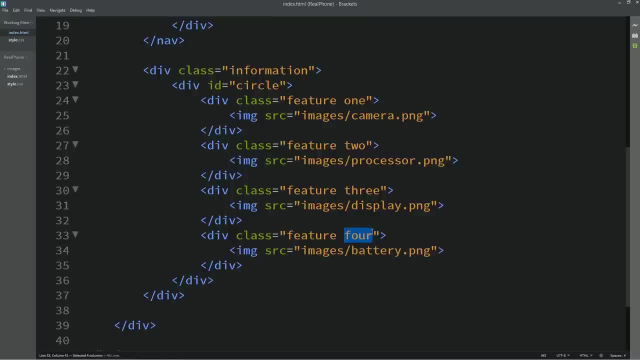 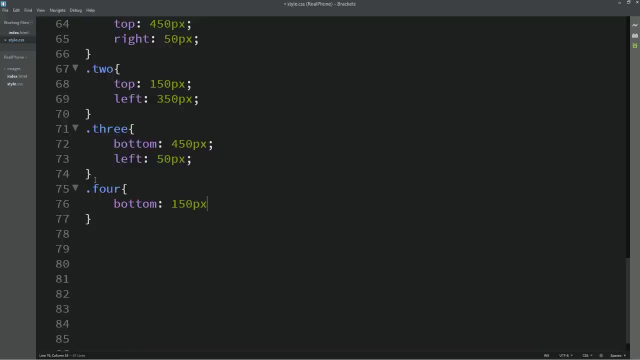 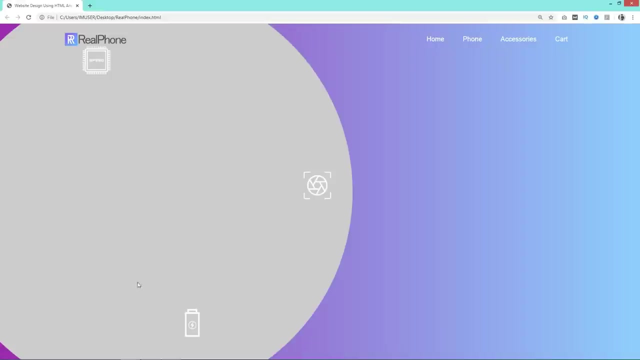 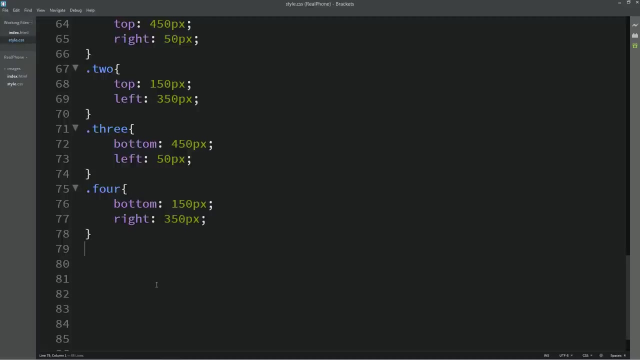 Let's write the fourth class name Here. I'm adding bottom and right. Save these changes, Then refresh the web page And you can see these icons at different position. One is not visible because that is in the left side. Now we'll add some content. 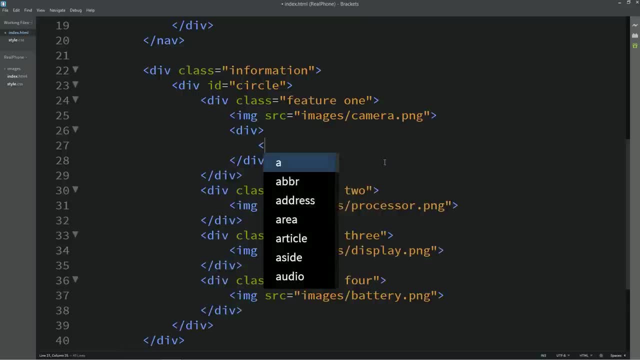 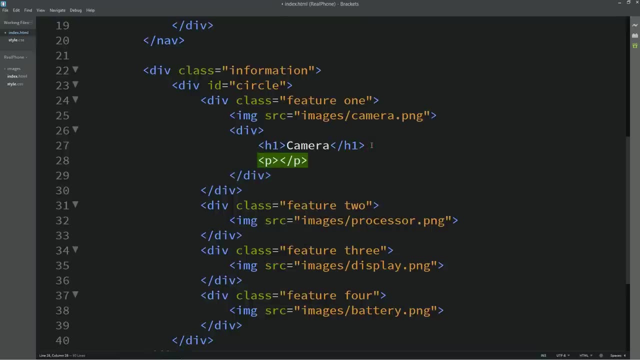 So let's come to the first feature Here. we'll create one div and we'll add title in h1.. So the title is camera. Next, we'll add a small text. So I'm using p And this is the text. So I'm going to add a small text. 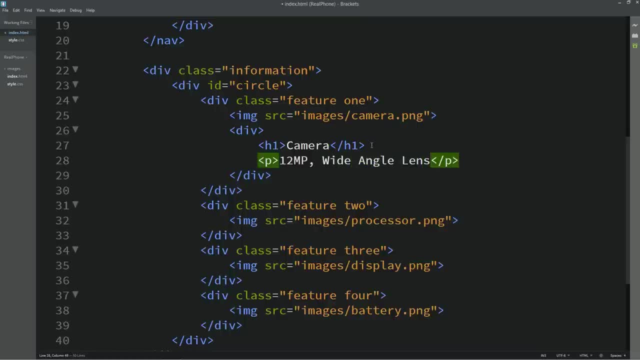 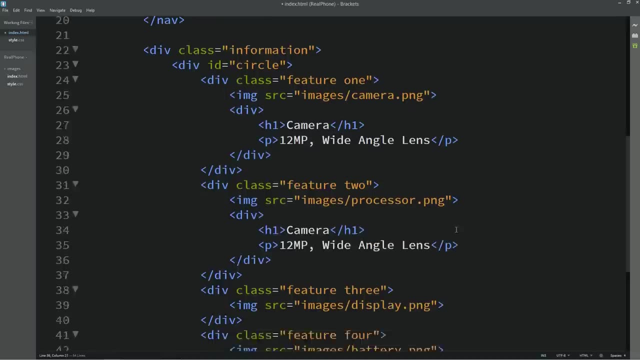 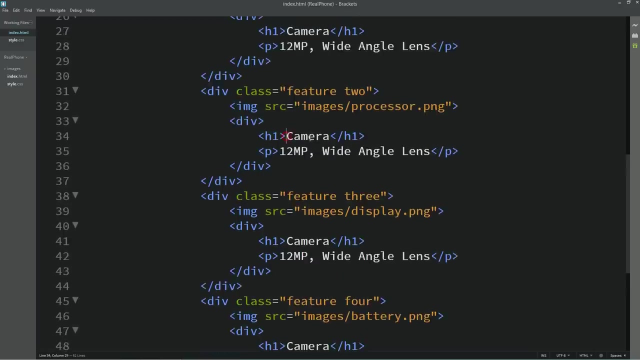 So I'm going to add a small text, So I'm using p And this is the text. Simply copy it and add it into the second one And for the third one and the fourth one, Then change the content. It will be processor. 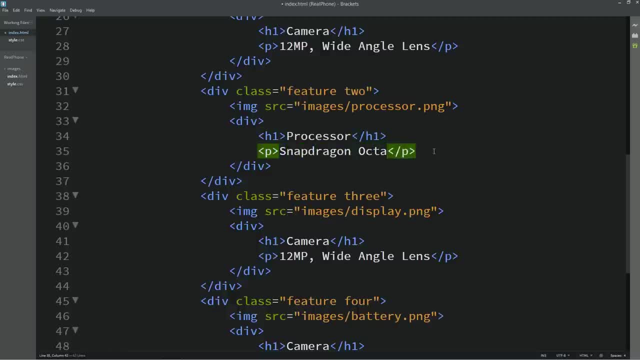 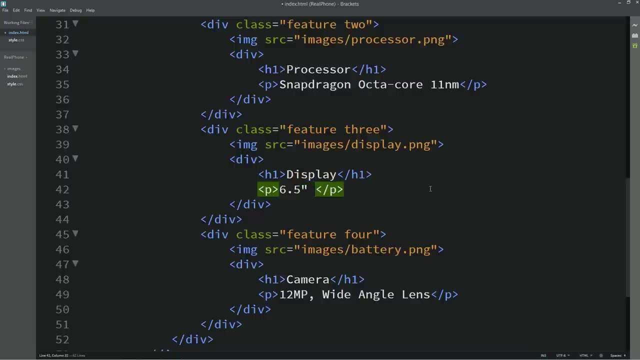 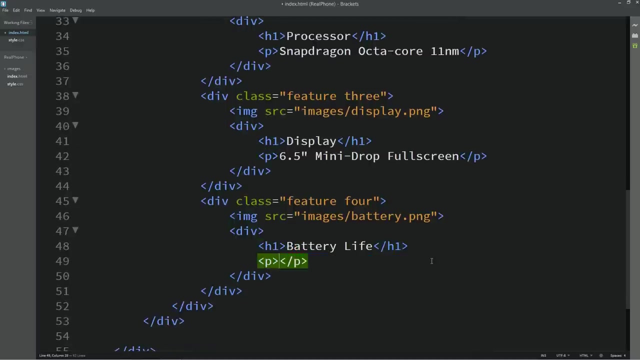 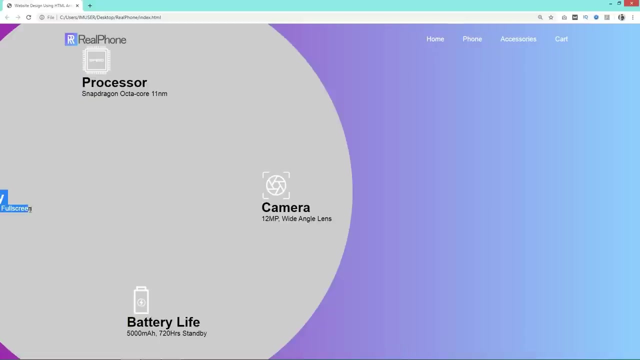 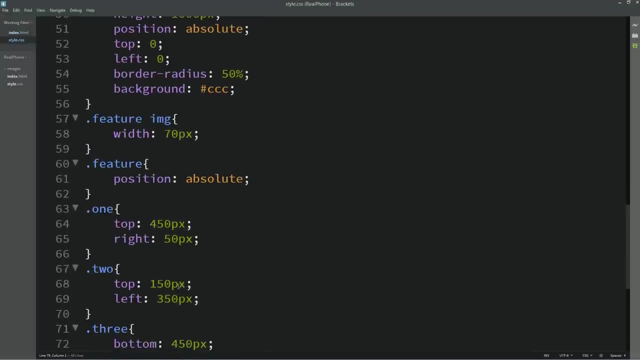 And we'll change the small text, also Change the content for the third one. Now for the fourth feature. It is battery life. Save it and refresh the web page So you can see one icon and some text below this icon. Let me come to this class name. 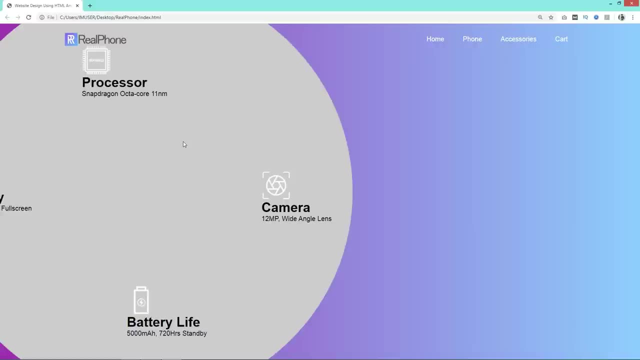 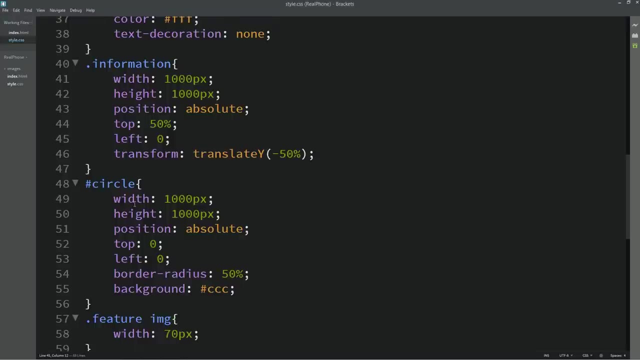 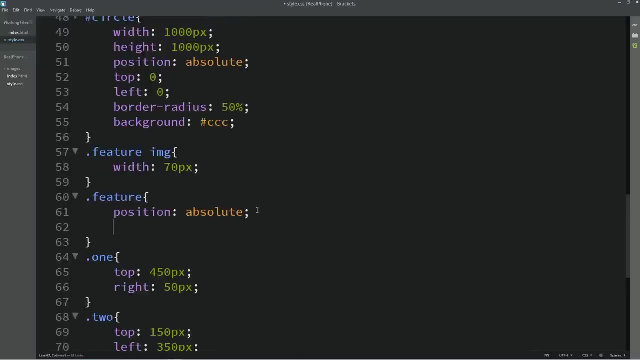 Information Here. we'll change it to Left 0. So that you can see all four icons here. Notice clearly: visual. Next we'll come to the feature and here we'll add display flex color: white. Reload the web page and you can see these text and icon in the same line. 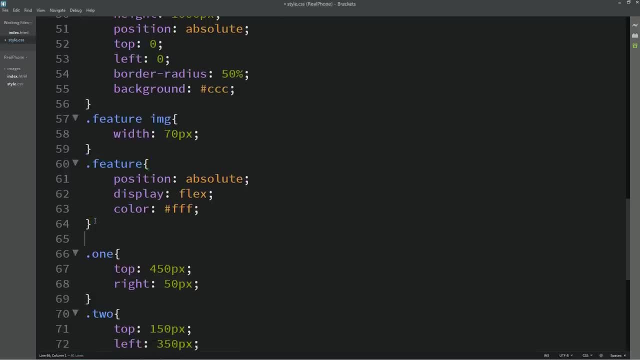 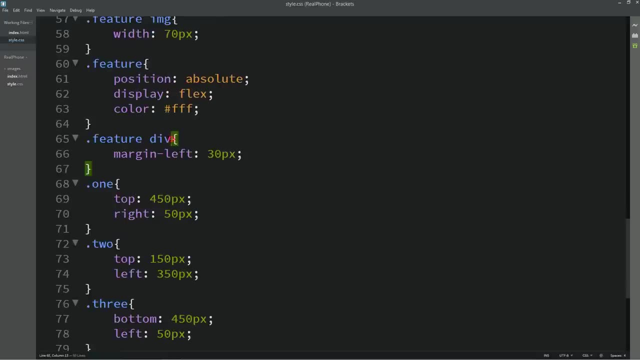 Just copy this feature and here we'll add div. We'll add margin from the left side. again copy it And here we'll add p for the small text. here we'll add margin, top reference to a page and you can see some space around these icons and around this small text. 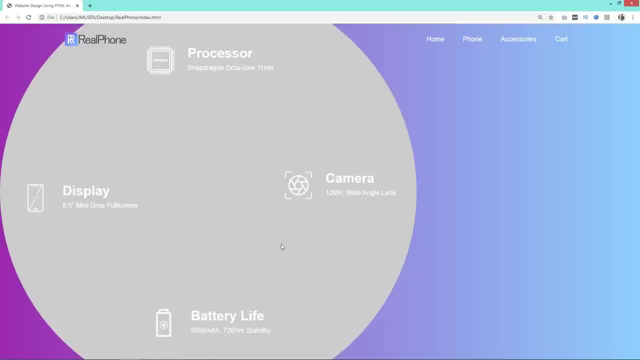 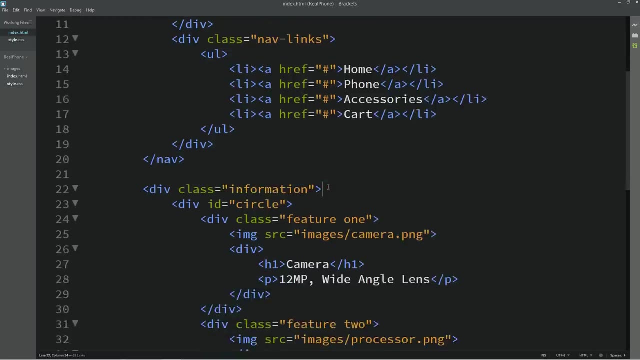 Here And we'll add it to the web page: See. Next we will add one image at the center. So come back to the HTML file and here we will add img source and the image file path. Let me add one class name for this image. 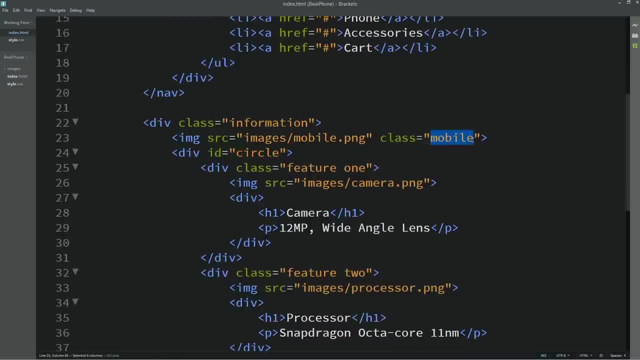 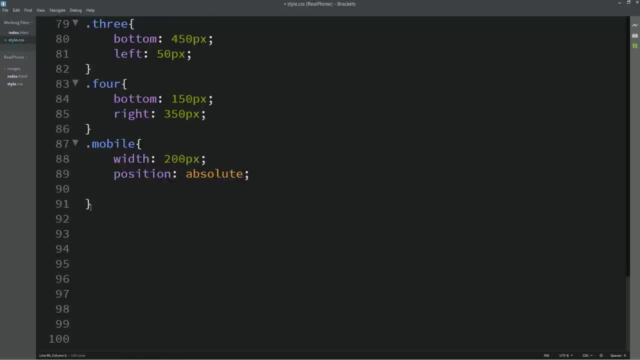 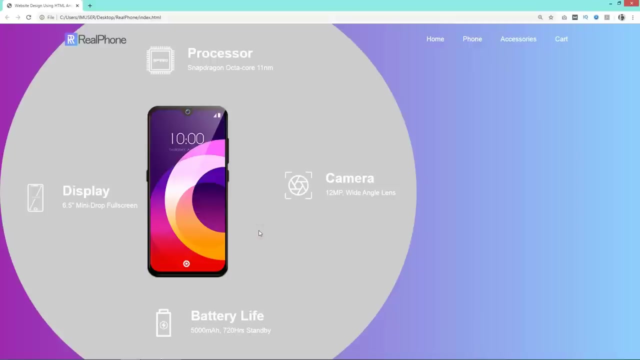 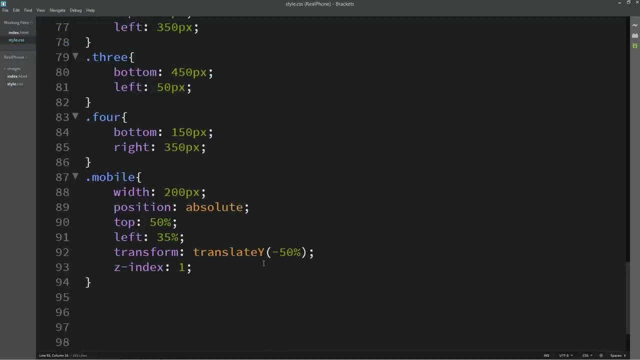 So I'm adding class name mobile. Use this class name in the CSS file here will set the width and position: absolute top left. transform. translate y minus 50%. set index one. refresh the web page and you can see this image at the center and some features around this image. 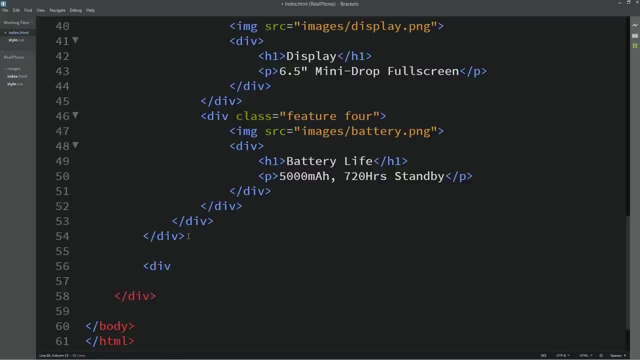 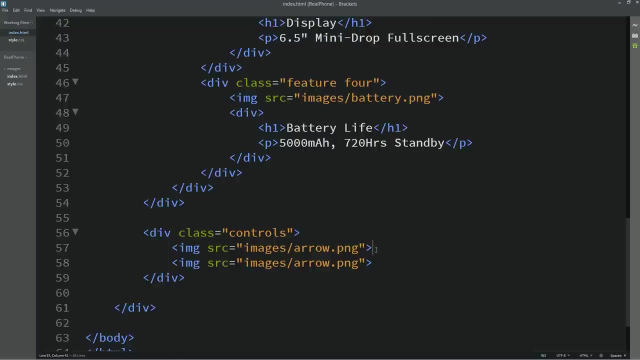 Let's come back to the HTML file and after this div will create one another div and here we'll add the class name controls. First we will add one up arrow, So I'm using IMG source and the image file path. Duplicate it because we need two arrows and between that will add one text. 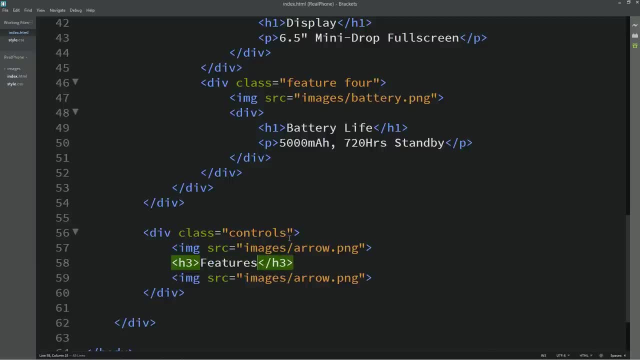 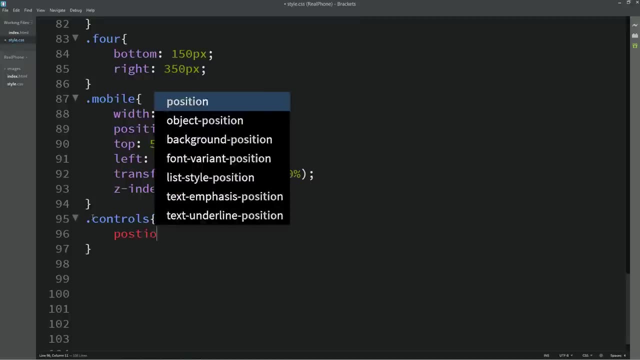 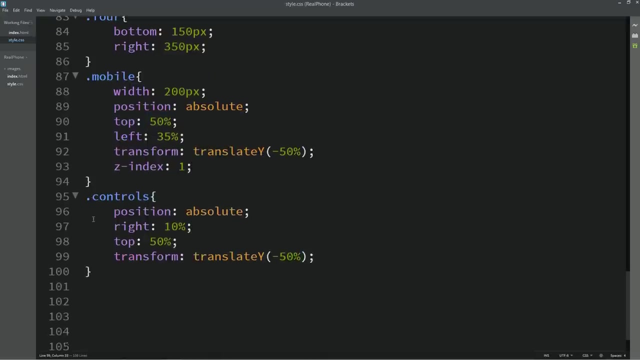 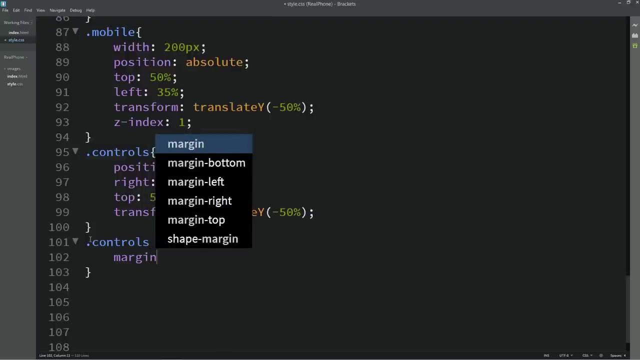 So I'm using h3 and the text is features. Let's copy it, Write it here in the CSS file and here we will set the position right top and transform, translate y. Let's copy it again. Then write h3, for the text here will add margin and color. 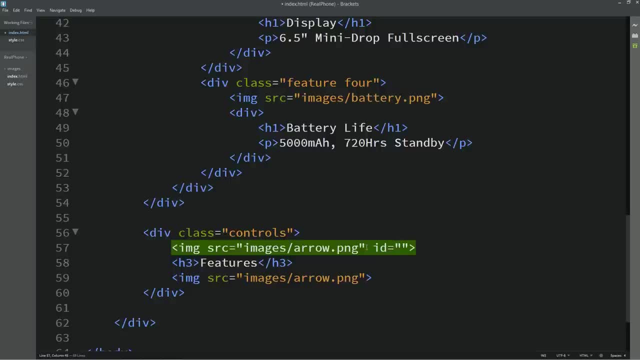 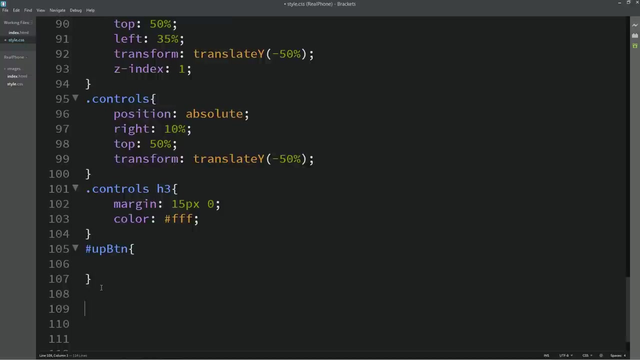 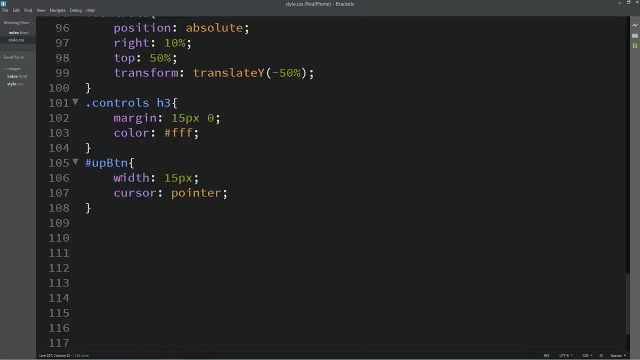 Let me add one ID. in the first icon It is up- btn and for the second one will add down btn. Let me copy the first one. I'll add it here. For this up btn. We'll add width And cursor pointer. 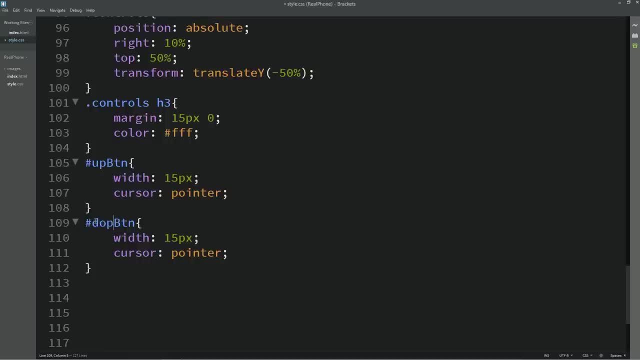 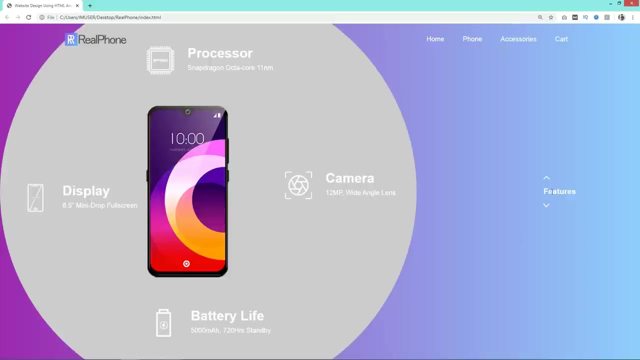 Simply duplicate it, and here we will change it to down btn. Everything will be same, but we'll add one more thing: Transform, rotate 180 degree. Now you can see this text and one up and down arrow. Let's come to the CSS file. 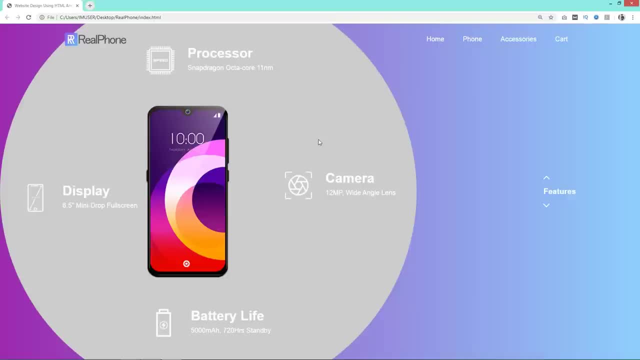 And in this controls We will add text: align center. Let's come to the CSS file And in this enter Reload the web page and you can see this icon in the center. Let's come back to the CSS file and in this circle, ID will remove this one. 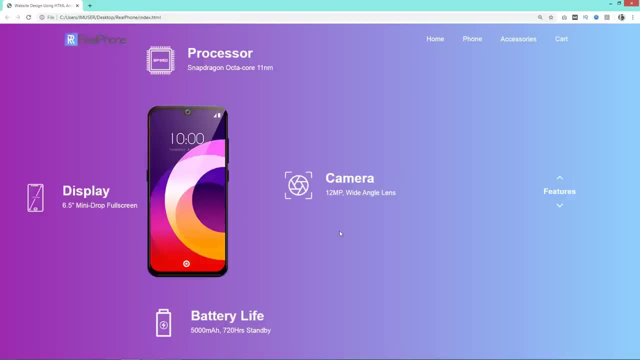 Save the changes and you can see this content here and this image. There's no background color for this, And next we have to add a click event for this up and down arrow. Let's add a click event for this up and down arrow. 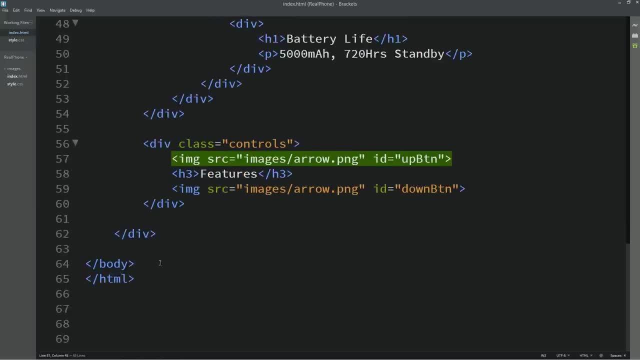 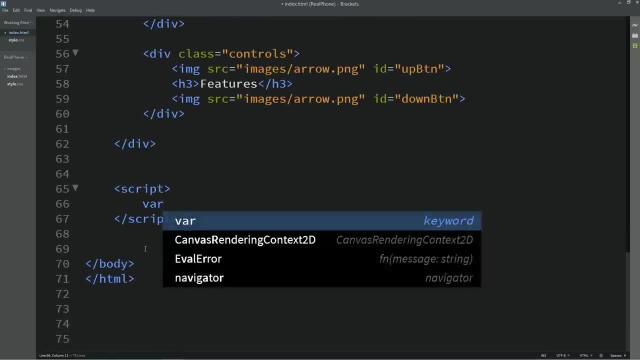 And next we have to add a click event for this up and down arrow arrow. so let's come back to the html file and come to the bottom, just before the closing body tag. here we will create a script, open and close, then create one variable name circle. 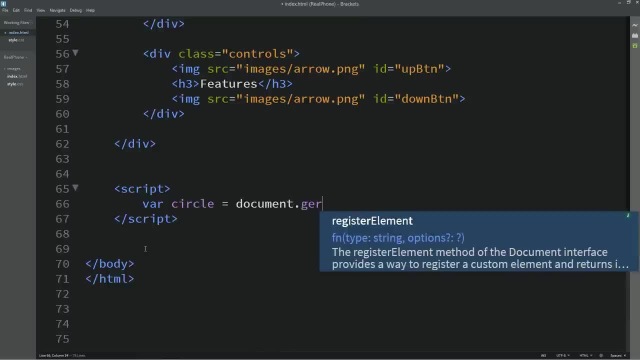 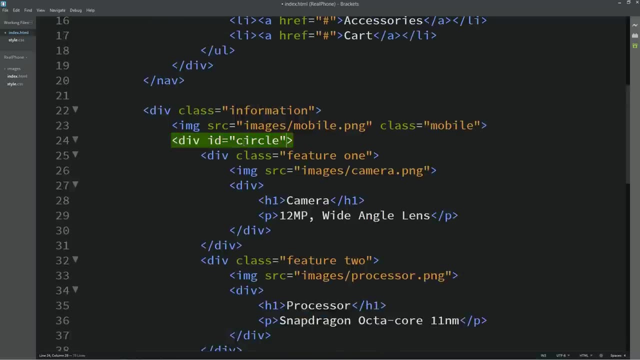 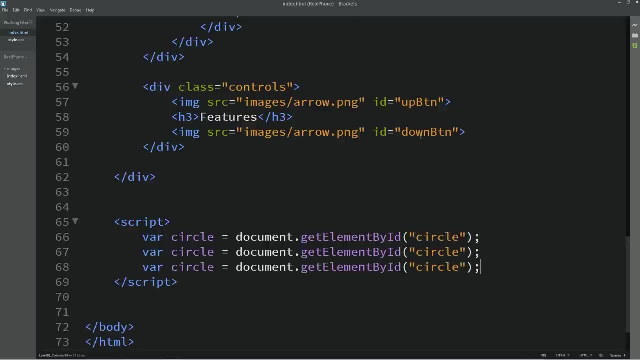 equal to document dot. get element y id, and here we will add this id circle. write it here, simply duplicate it, and in the second one we will add this one: upbtn, and here also upbtn. now for the third one: downbtn and variable name: downbtn. 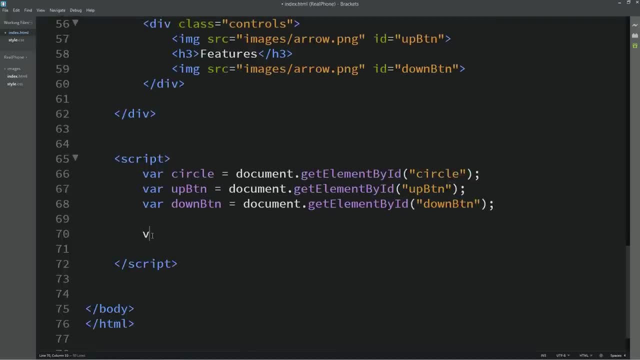 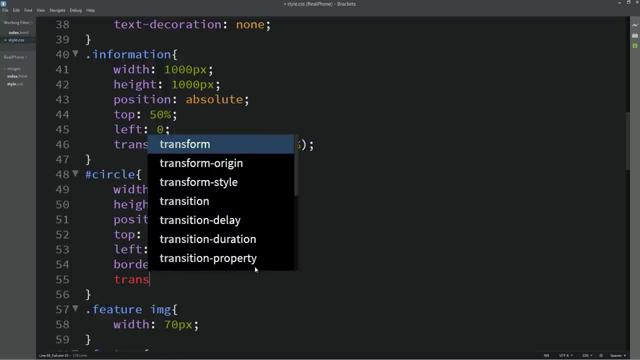 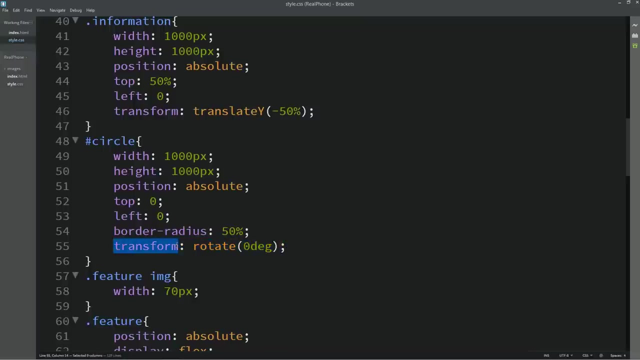 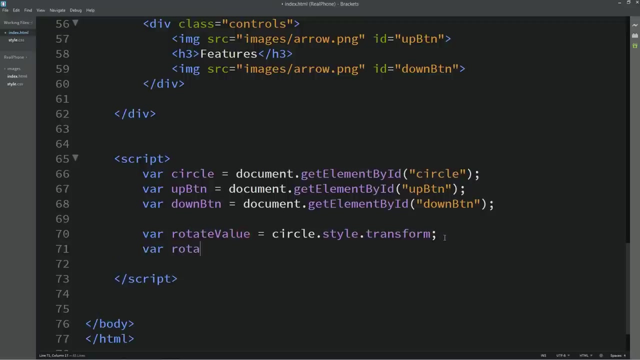 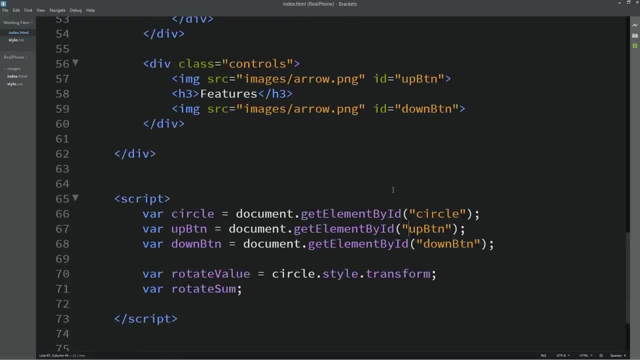 let's add one more variable. rotate value is equal to circle dot, style, dot, transform. So first we will add one transform: rotate zero degree. So right now it will store zero degree in this variable. Let's create one more variable here: Rotate some. next will add: click event on this button. 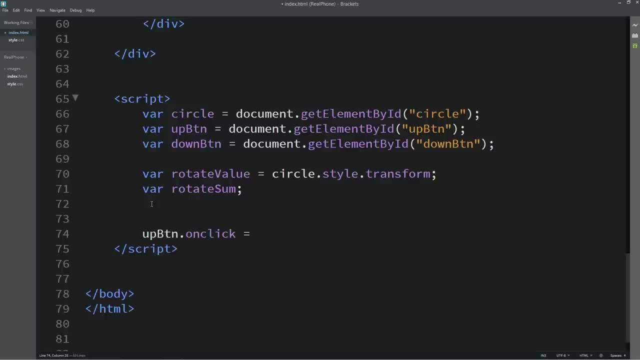 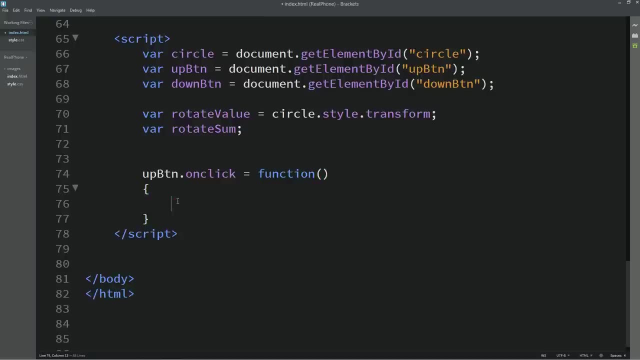 So here we'll add up btn dot on click equal function. In this function we will add rotate, some equals rotate value plus Rotate minus 90 degree, because it will rotate the content in anti-clockwise direction. So suppose initially if the rotate value is zero, so it will rotate the content by minus. 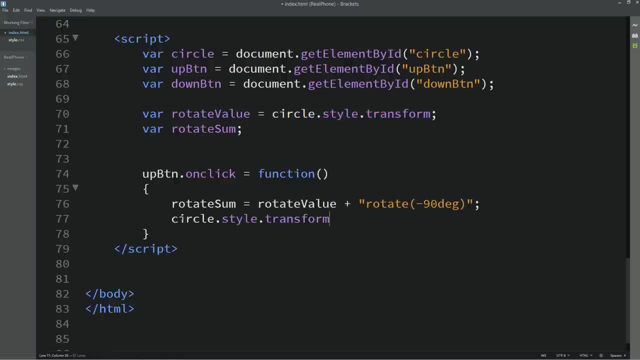 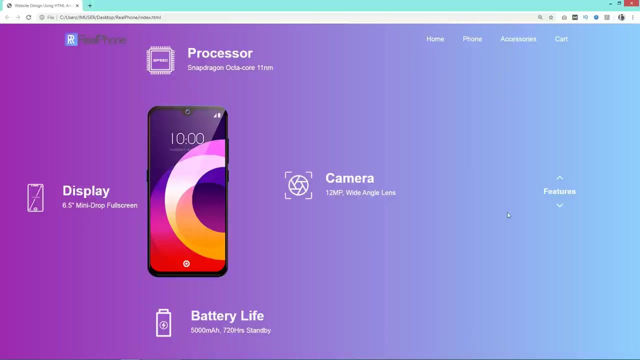 90 degree. Next, just copy this one circle dot style: dot transform equals rotate some. Then we'll add rotate value is equal to rotate some, So it will update the Existing rotate value is equal to rotate some. Save these changes and reload the web page. 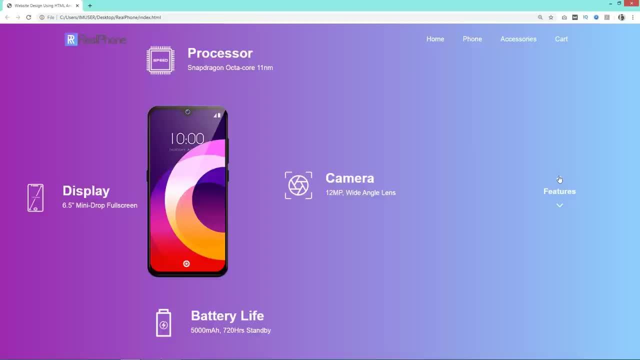 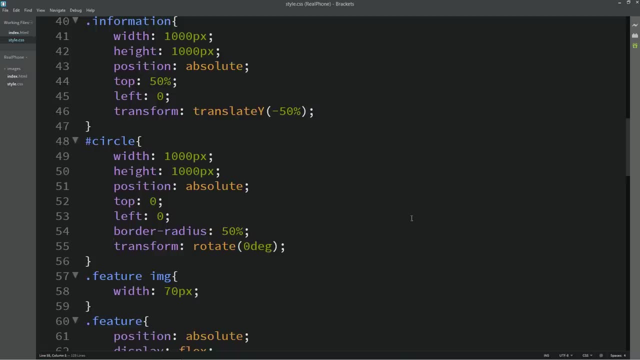 Now you can see. if I will click on this up arrow, it will rotate the content in anti-clockwise direction. It is rotating very fast. We need to add some transition. So just come back to the CSS file. here We will add transition one second. 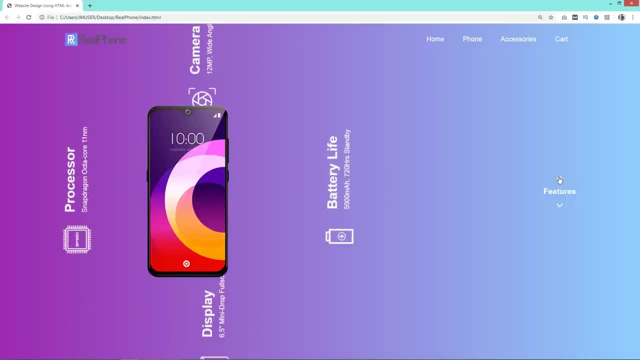 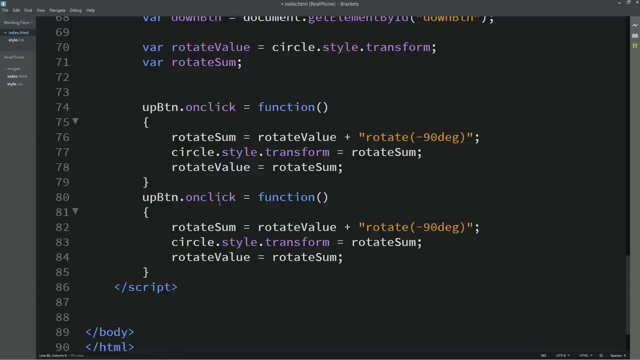 Then refresh the web page and you can see when I click here it rotate the content in anti-clockwise direction. Right now you can see down arrow is not working, So we'll add the same concept in the down btn. Just copy it again. 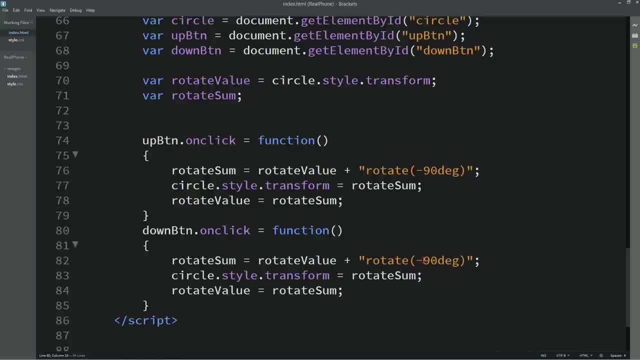 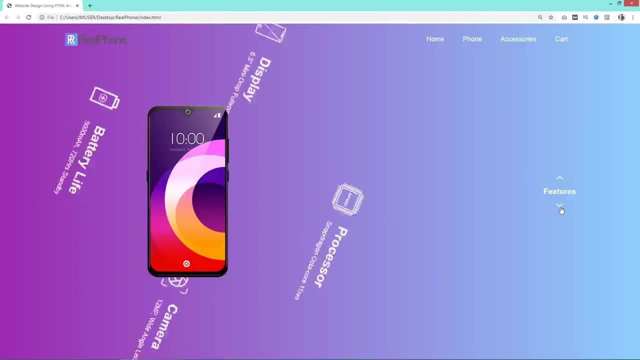 Here we'll add down btn And it will become plus 90 degree. That's it. Reload the web page. You can see when I click here it will rotate the content in clockwise direction. Next we have to rotate each content of this phone features. 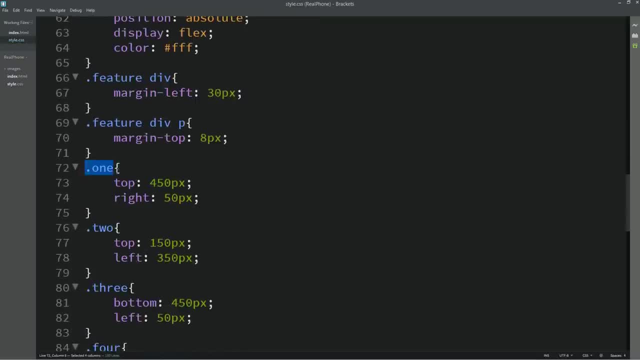 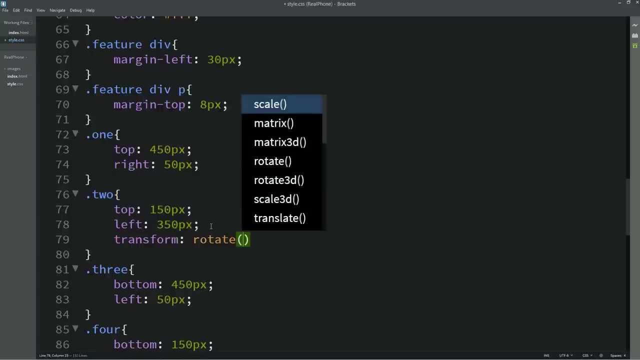 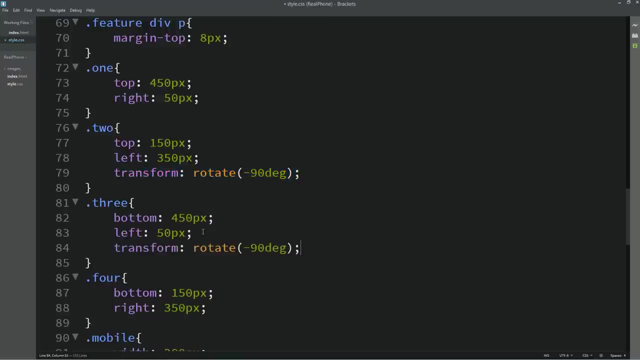 So just come back to the CSS file, and here in the second one we'll add transform rotate minus 90 degree. Just copy it and add it into the third one. It will be rotate minus 180 degree. And for the fourth one, 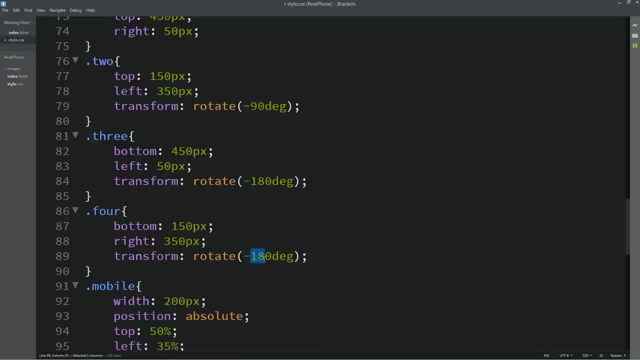 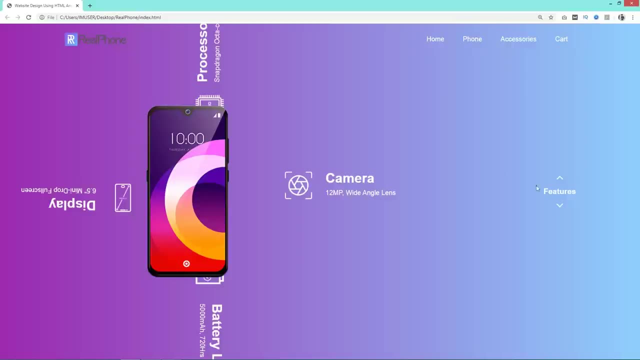 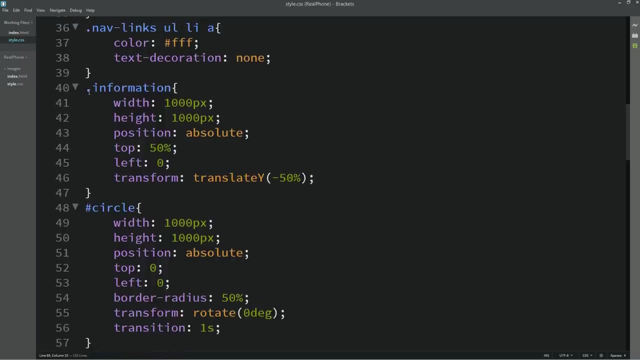 It will be minus 270 degree. Refresh the web page And you can see when I click here In the right side, it will display horizontally. Next I will move it into the left side. So just come back to the CSS file and in this information again, we will change it to minus. 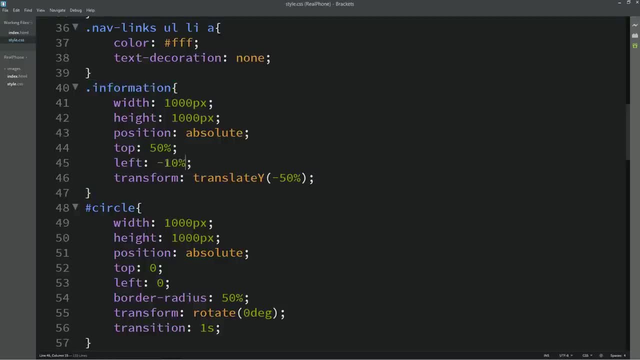 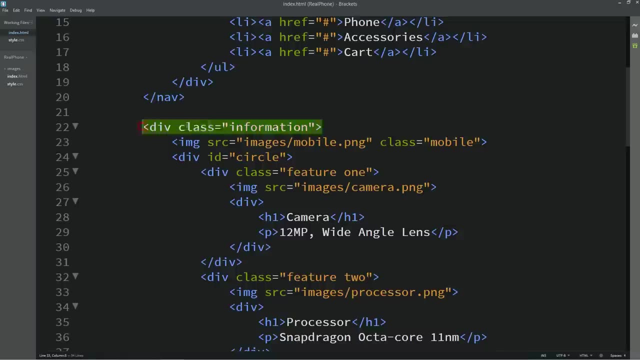 10%, And next we have to hide, So we will add the size. It will also be 9.. It will be 8.. We will also need to change the font size And we will add the font size to our font size. 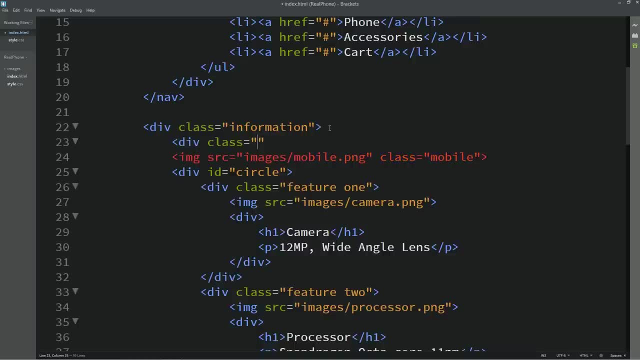 So we will add 1 font size And we will add 1 font size and we will add 2 font size. We will also need to add 2 font size And we will add 3 features of this phone and only one feature will be displayed. 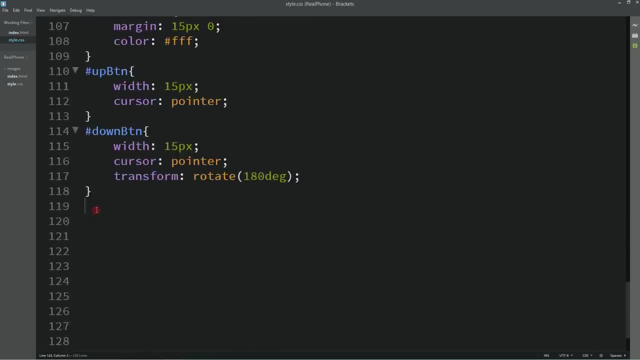 So just come back to the HTML file And here we'll add one div And the class name I am adding overlay. That's it. There is nothing in it. Just copy this class name overlay, write it into the CSS file. Here we'll add width 0 and height 0.. 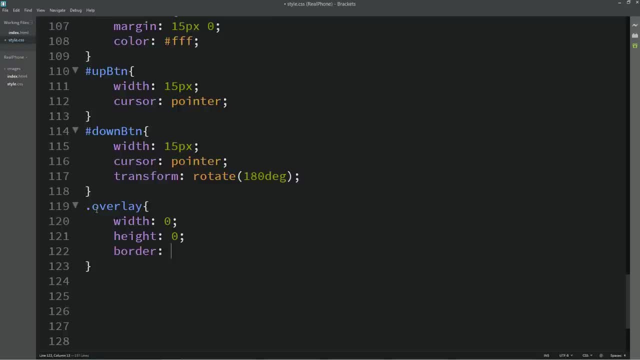 Next, we'll add border-top- 500 pixels- solid White color And we'll add a line: border top- 500px- solid white color. simply duplicate it and it will be border right, it will be border bottom and it is border left. next, we will change the color: it will be red. 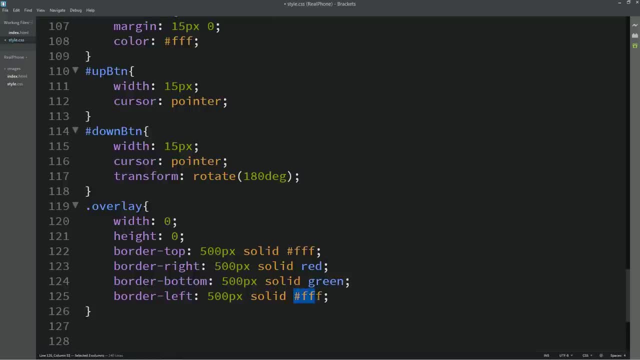 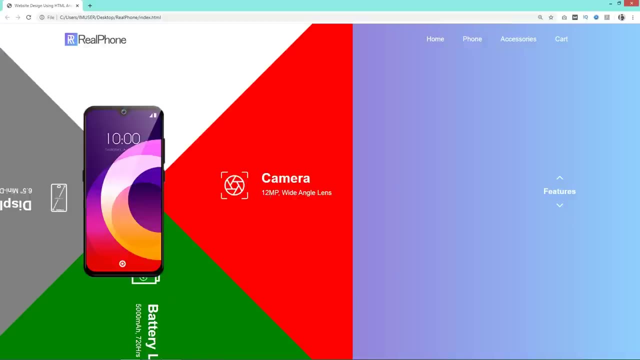 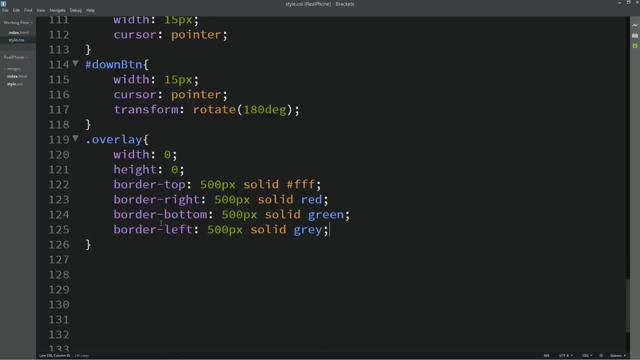 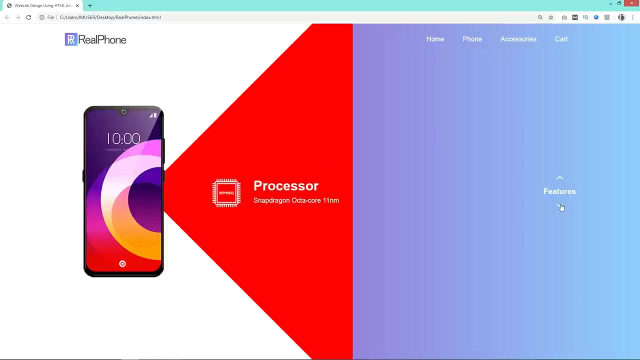 it will be green and this one gray. so that you can see how it works, you will see different color in each sides. next, we will add position absolute left 0 and top 0 and we will change this color. it will be white and this one also white. 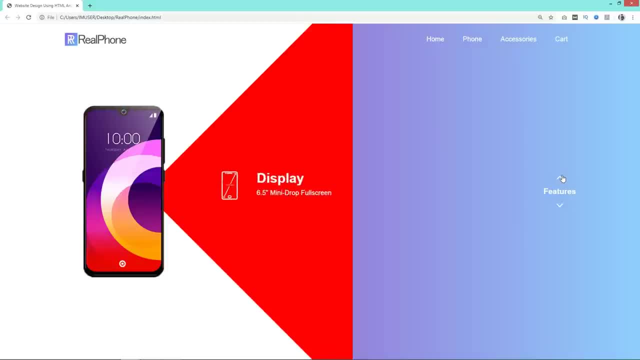 so that you can see only one feature right now. so So let me change it to transparent, refresh the web page and now you can see only one feature in the right side and other three are hidden, and when I click on this button, it will rotate the content and display the another feature of this phone.